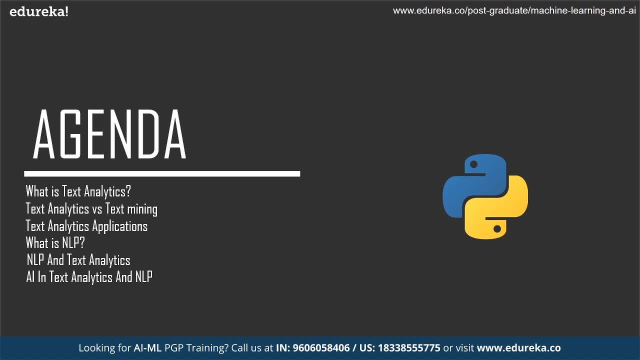 of the session. guys, in the next session We will work on a few projects to understand AI in text analytics. Also, don't forget to subscribe to Edureka for more exciting tutorials and press the bell icon to get the latest updates on Edureka. and do check out Edureka's. 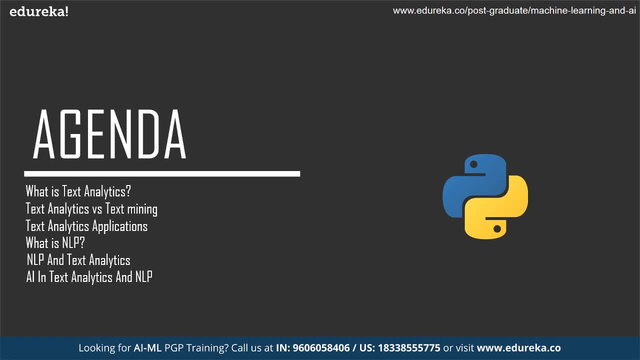 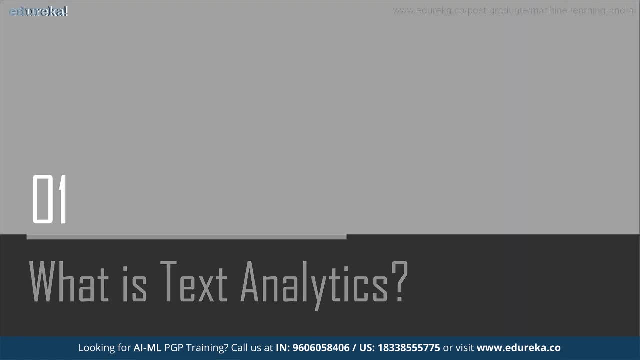 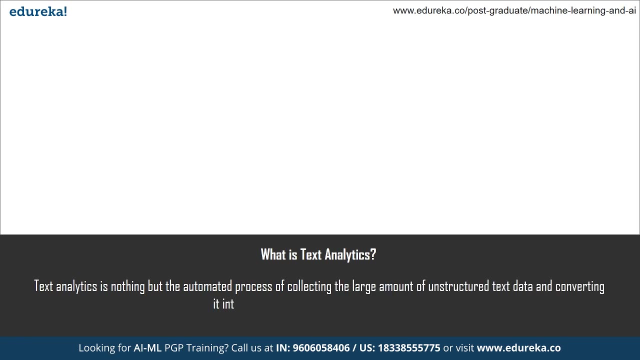 postgraduate machine learning and AI certification program. The link is given in the description box below. now, without any further ado, Let us understand what is text analytics and how to use text analytics. Text analytics is nothing but the automated process of collecting the large amount of unstructured text data and converting it into quantitative data, which 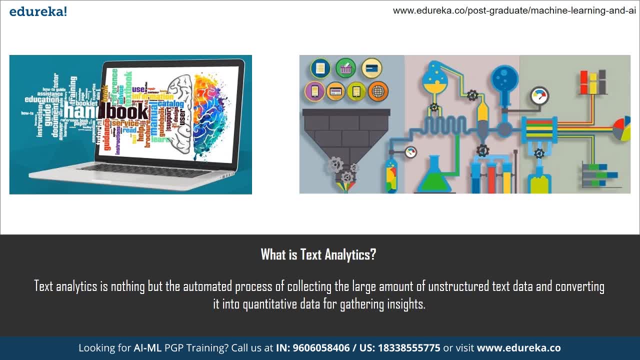 eventually helps in understanding patterns and uncover various trends and insights. So we can combine this data with visualization tools and make decisions based on the insights for the greater good. the main objective of text analytics lies in why we actually do it, So we'll take a look at. 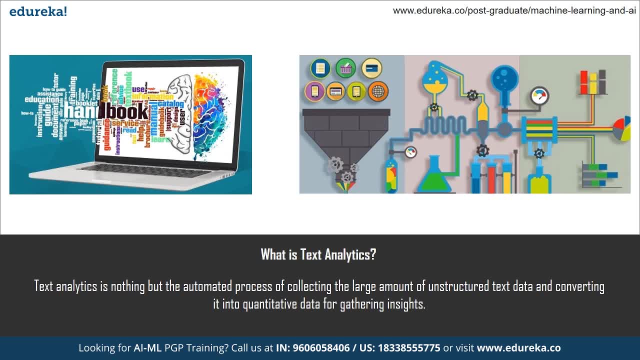 Why we do text analytics in the next part of this session, But before that, let me give you a clearer picture of what text analytics actually is. So if I take the example of our social media platform, let's say Facebook or Twitter- there you can see a lot of post with a lot of textual data that can be used for, you know, identifying 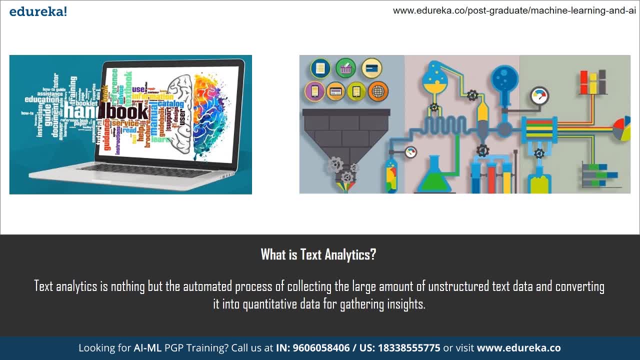 a set of pattern, or it may help in understanding trends or insights. you know the kind of times that we get in hashtags or the trending topics, So these are actually found by doing the text analytics on very large unstructured text data which we convert to, you know, quantitative data. 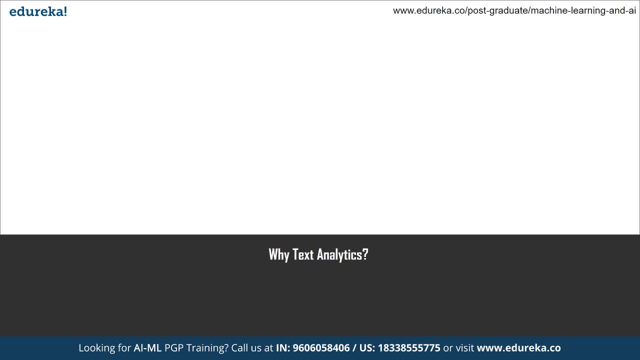 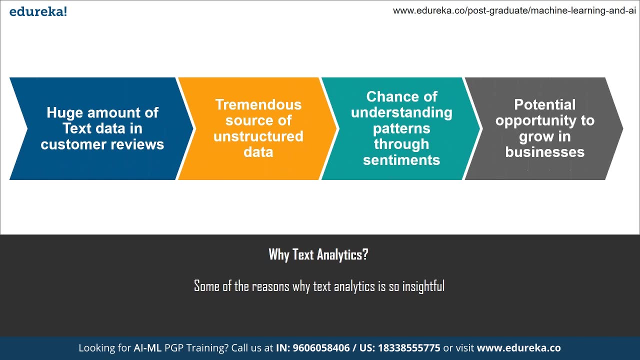 and it helps in understanding the patterns guys and taking a look at the main objective, which is why we are doing this. All right, So let's go ahead and understand why we are using text analytics, followed by a few applications and examples as well. 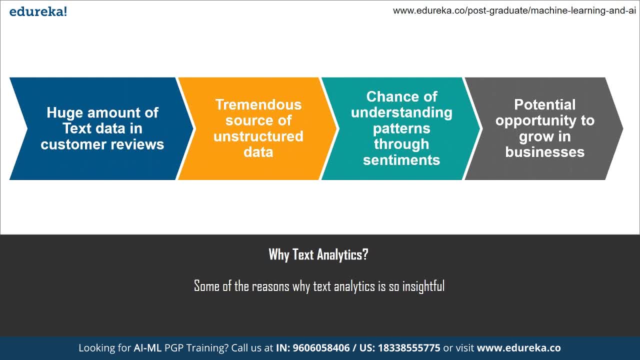 So I'm sure most of you must have come across a feedback space. you know, whenever you go to a website or do something on a new app or install a new application on your mobile, You always see a feedback space where a customer is expected. 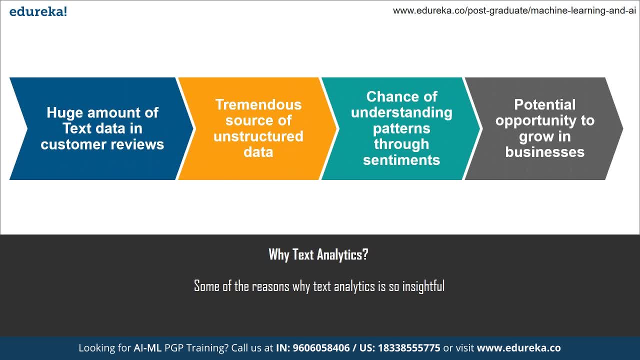 to share their thoughts about their experience. It may be anything, guys, and this is not just limited to restaurant review or video quality on a streaming platform. The written communication plays a very important role in every aspect of human civilization, and governments, educational institutions and social media platforms are flooded with an unstructured text data. 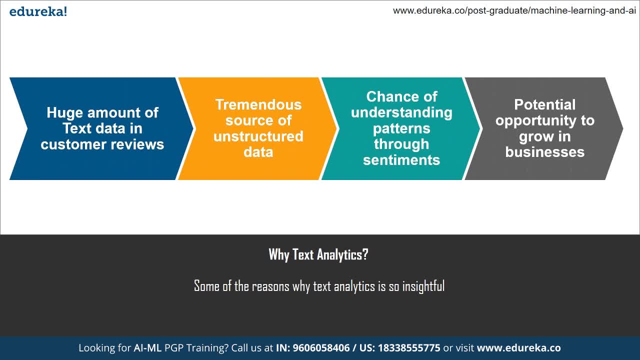 that we can actually gather, collect it and use it, Change it or, you know, transform it to use for our own best. the need for the text analytics has emerged with the digital Revolution and Advancements in the fields like machine learning and artificial intelligence. now, with the technology and the tools that we have, we can use this unstructured data. 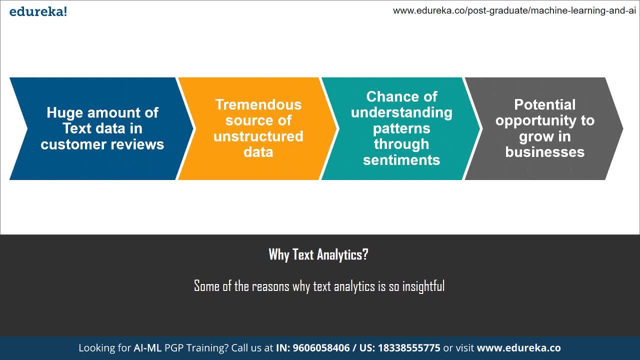 to understand patterns in behavior, in decision-making, in opinions, intelligence, etc. businesses mostly do it to understand the negative reviews and to rectify The customer needs in a way to make a greater impact. It is quite evident that the text analytics is quite efficient and important sometimes text communication patterns. 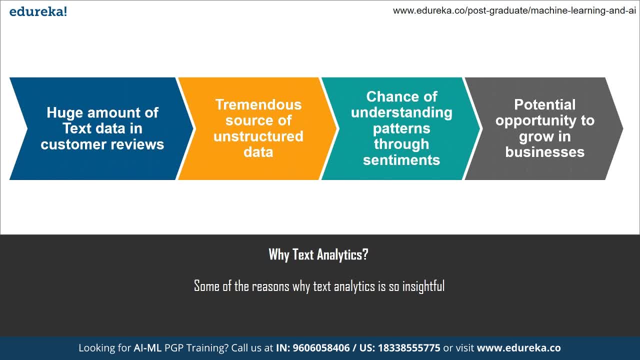 can drive a lot of insights. when I say inside, it is the solutions you know, the ideas that you get after the text analytics, It can actually give you a lot of insights about how a person is thinking. more importantly, with text analytics We can unlock the very needs. 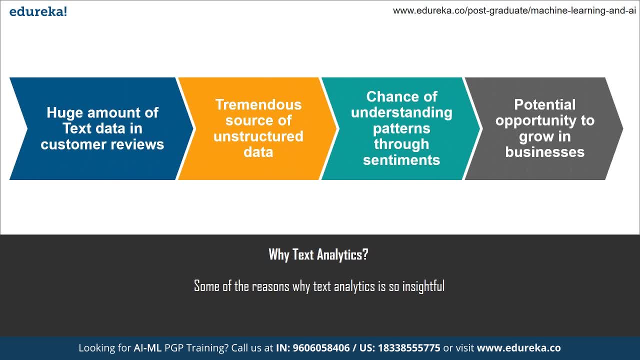 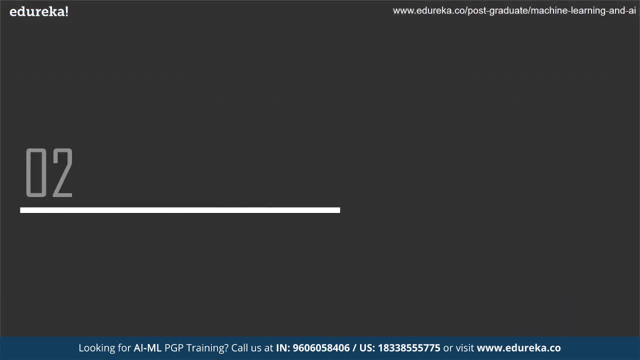 and demands of the customer to grow the businesses. and you might come across the term text mining often when you start reading about text analytics. So let us take a look at the difference between text mining and text analytics. So there is a very basic difference between text mining. 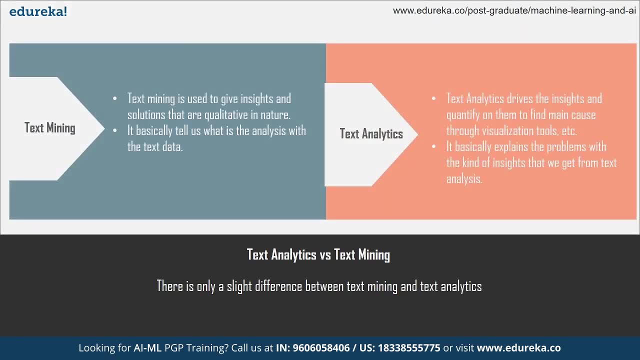 and text analytics, that is. you know, text mining is often used to give the solutions or insights that are qualitative in nature. So if you are doing a text analysis or text mining on something, So let's say you're trying to do text analysis on our e-commerce website. 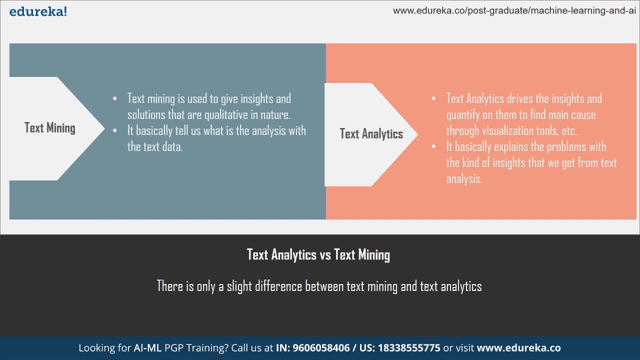 where you want to check the reviews So you might be able to get a qualitative perspective, where you might get the reviews in the shape That is, a good review, Maybe a bad review, or a very, very good review, or an excellent review- and, on the other hand, 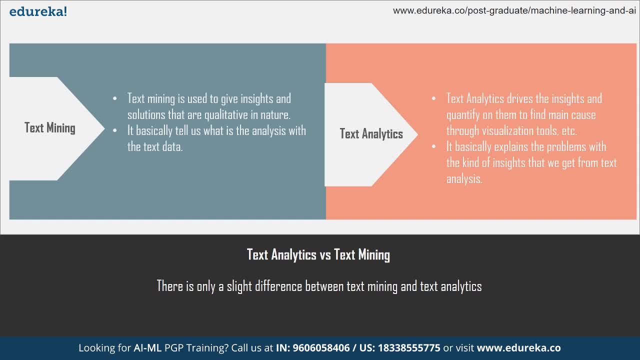 a text analytics magnifies these results or the insights that you are getting into a way to find the main cause or the problem through many visualization tools. So basically, text mining will tell you what is wrong and text analytics will tell you why it is wrong. 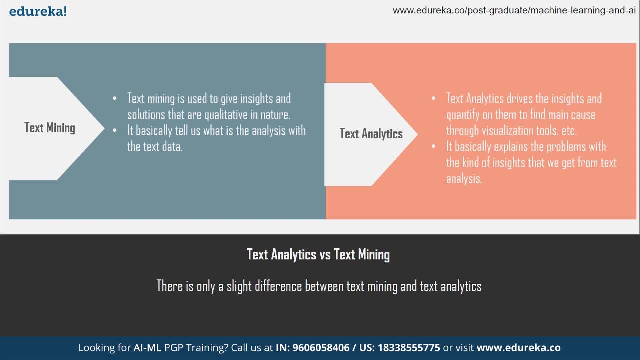 in the first place. So, taking example of the e-commerce business, when you do the text mining on it, you get the qualitative perspective in which you get several answers like good, bad and very good, excellent, Etc. But with text mining you will be able to identify: 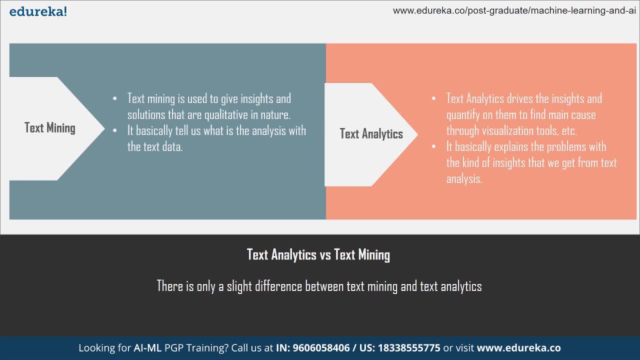 for all the bad reviews. What is the reason or what is the basic thing that you're lacking, so that you may be able to improve there? So that is the difference between text mining and text analytics. Now let us go ahead and take a look at a few applications. 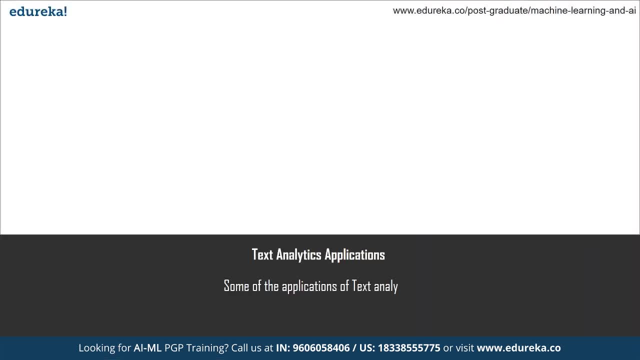 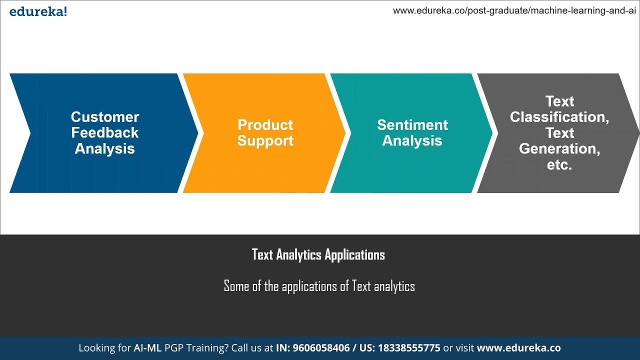 of text analytics guys. So the first one is customer feedback analysis. So I'm sure most of you have heard about a customer feedback, So it's usually a sort of opinion or your experience review that people actually ask in a lot of e-commerce website after the shopping. 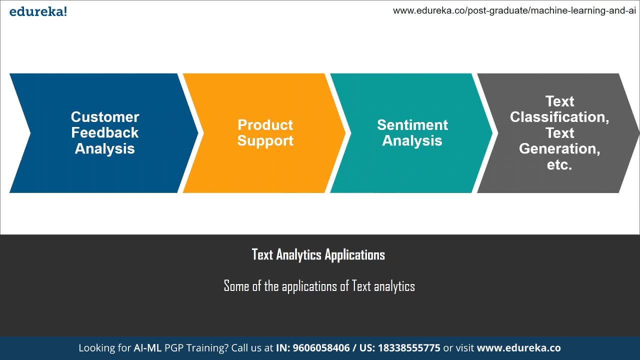 They ask you for the experience and if you have faced something that you don't like, they will ask you for a feedback as well. So customer feedback analysis through text analytics basically points out various shortcomings gathered through processing the customer reviews. So let's say you have 5,000 customer reviews. 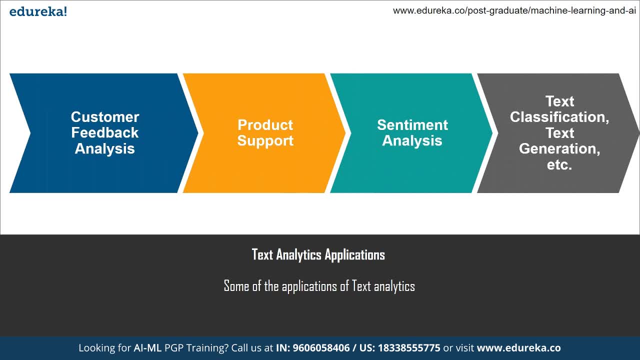 and to find out how your customer are liking your product, or anything for that matter. You will be able to do the text analytics and, based on the insights that you're getting, you will be able to point out to exactly what's wrong or what is actually benefiting you, so that you can grow. 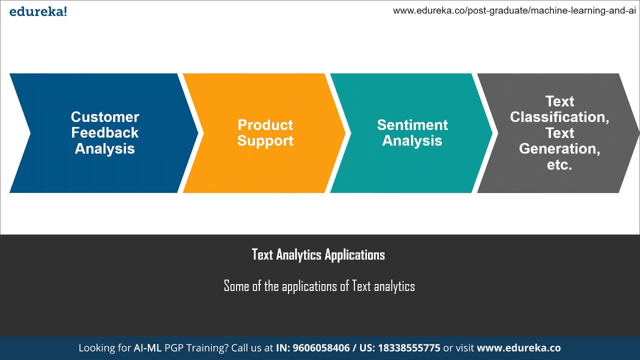 into your business, Etc. And next up is customer service as well. So using text analytics to analyze the content of support tickets, for example, can help you understand your customers needs. So when I say customers needs, you will be able to analyze through all the set of patterns or the tickets. 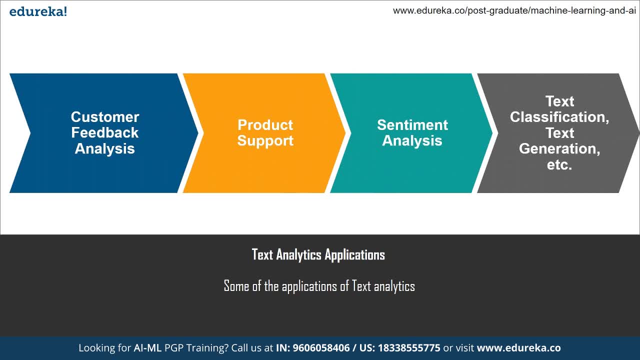 that you're getting, you will be able to understand what your customer is really asking for. So, over there, true text analytics, you will be able to identify the demand So that you may increase your supply as well. You will be able to identify those points as well. 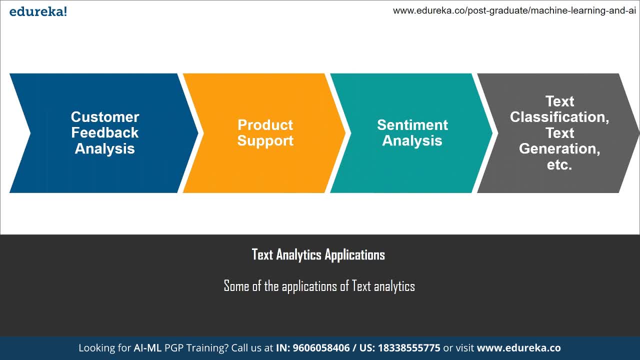 in which you may need to work a little harder or a little lesser to your balance out the business, and you can actually gather motivations and expectations as well through this support tickets and by text and analytics, and it eventually provides you the insights to rethink your customer experience strategy as well. 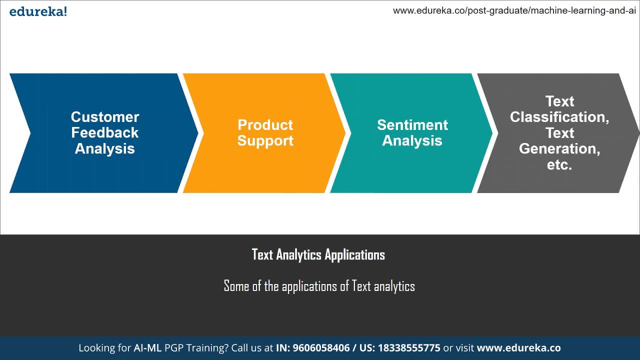 And next up is sentiment analysis, guys. So sentiment analysis: It helps in identifying the emotion behind the text, and with text analytics It can be further narrowed down to those needs and shortcomings that will eventually change the sentiment if needed, and a simple example would be analyzing: 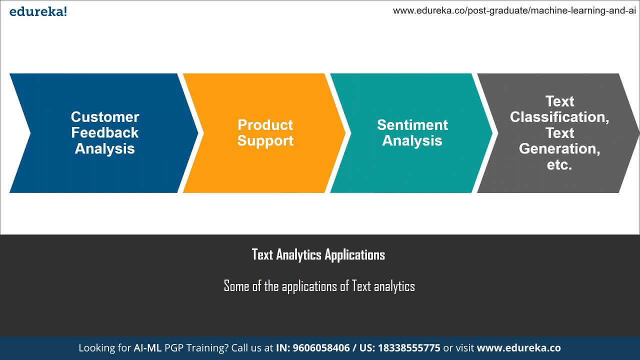 the social media post about a particular product and through sentiment analysis We get the most common emotion and then we can quantify on it by decision-making based on the analysis. So the text analytics solutions You give us the problem with the product or anything that is going on good. 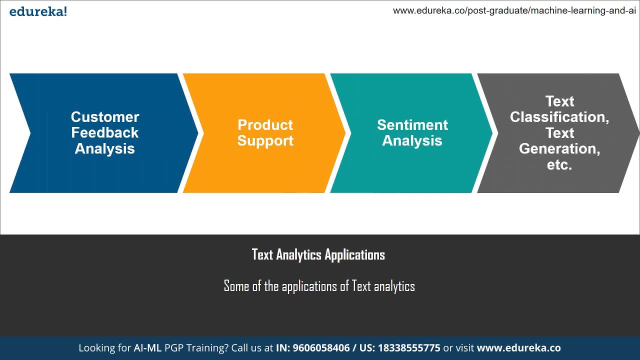 so that you can quantify on the good things as well, or a suggestion to make it better with insights. These are only a few applications of text analytics, just to give you a perspective of what really is going on. And now that we know about these few applications as well, 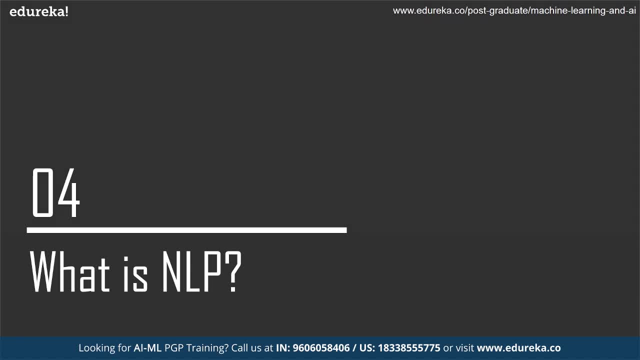 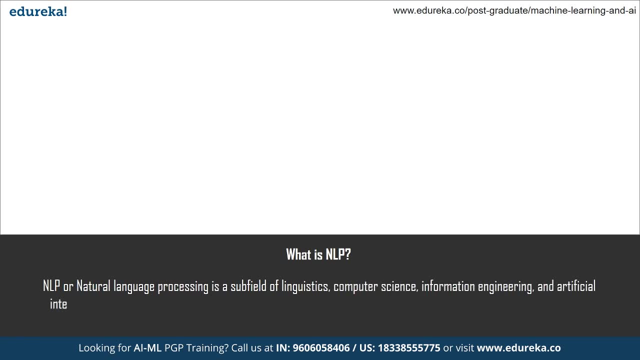 Let us take a look at what is NLP, or natural language processing. So to understand natural language processing, or NLP, We first have to learn about natural language. so natural language is nothing but how the humans communicate with each other, and it is nothing but the communication through text. 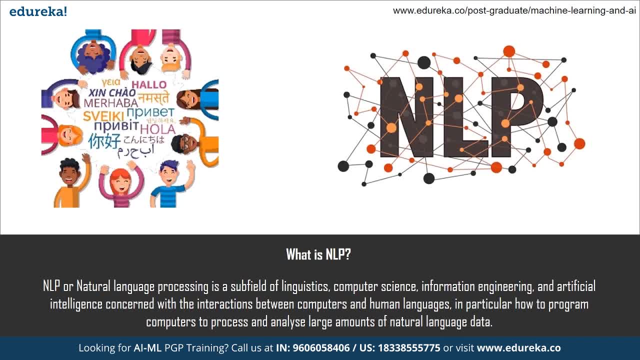 It could be a communication through speech as well, And these are the most common communication techniques for human now, since we know that there is a lot of things we can determine by the way somebody communicates with you. So this was the main objective of the natural language: processing to process. 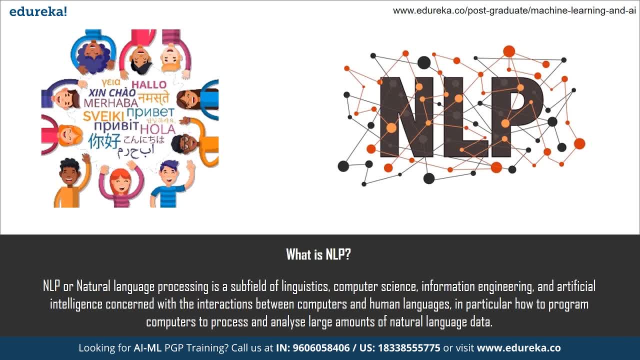 this natural language data, That is, the text data and the speech data. So naturally, this process faced a lot of challenges, including a lot of linguistic barriers, since the way of communication changes demographically from region to region all across the world and, for example, 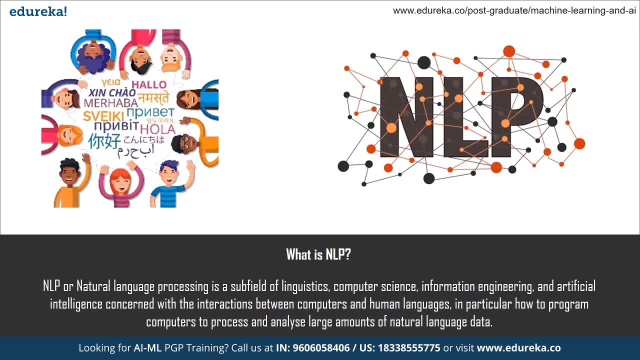 like in English, we agree people by saying hello. in Spanish It becomes Ola and thank you becomes gracias and like that, you know. and to process this natural language data, other challenges included unstructured and most of the times the data was quite incomplete. 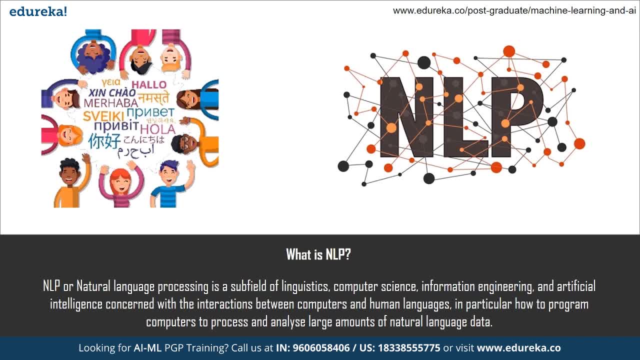 And if we go by the definition, natural language processing is a subfield of linguistics, computer science, information engineering and artificial intelligence concerned with the interaction between computers and human language, in particular how to program computers to process and analyze large amount of natural language data. So when we look at it from the text analytics perspective, 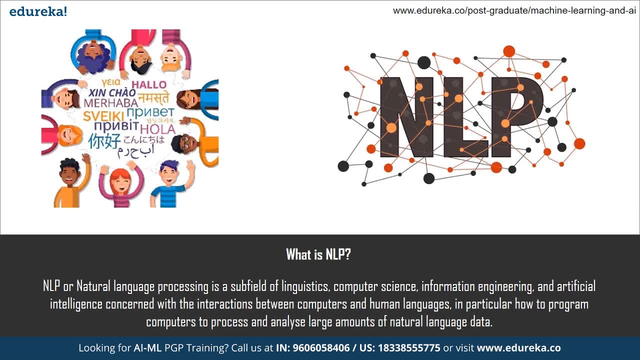 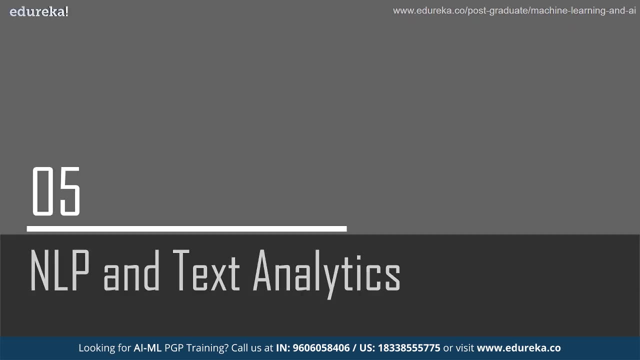 basically, what NLP is doing for us is helping us to load the data So that the computer is able to understand the text data. So now that we know what NLP, or natural language processing is, let us take a look at how NLP and text analytics are connected together. 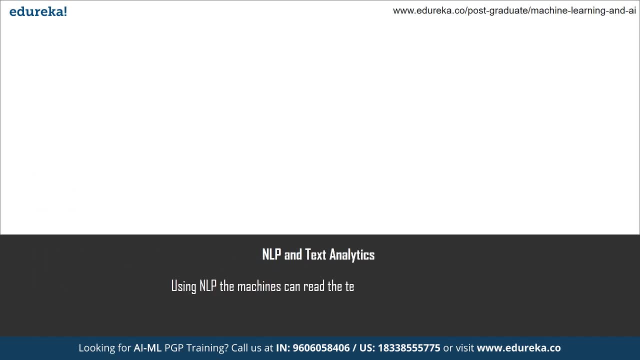 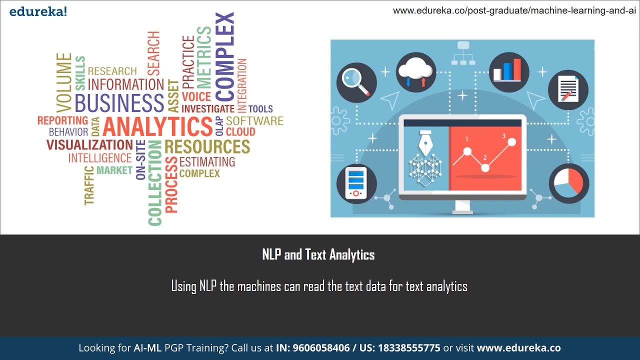 So NLP is basically a very important component of text analytics. It is used to basically make use of NLP algorithms for linguistic analysis or analysis of natural language, which in our case is the text data. It could be the speech data as well. 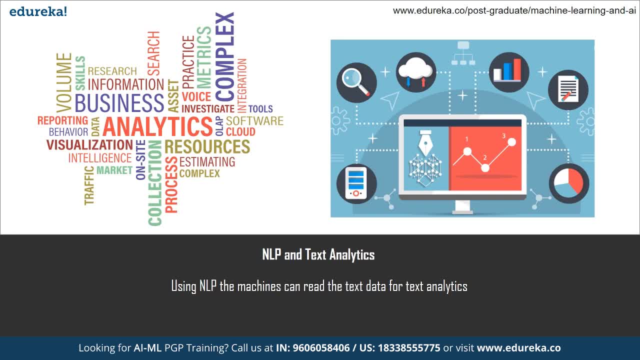 but we are only using it for text data in text analytics and using NLP, the machines are able to read the text data for text analytics, obviously, and one of the example of how NLP helps in our text analysis is how it actually helps in identifying irrelevant keywords. 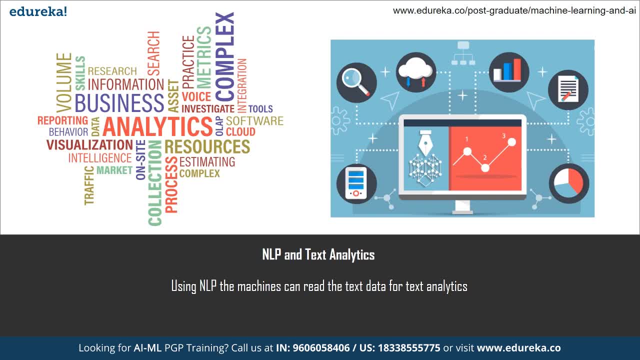 in search engines like Google. So a lot of spam that once used to rank on the search engines just by stuffing more keywords and are basically now identified through text analytics and NLP. so earlier, Whenever you wanted to, you know, rank your content, You just used to stuff it with keywords. 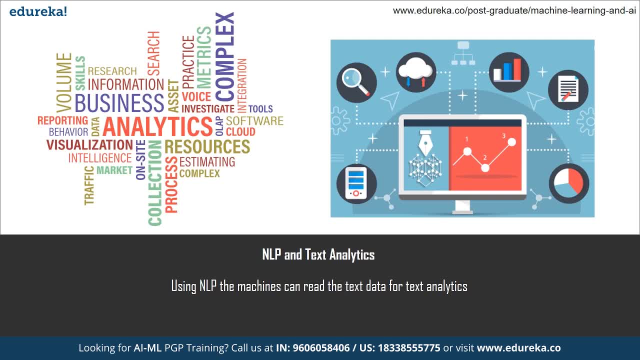 that are high ranking keywords. But now, with text analytics, search engines like Google are able to identify spam content because they are able to analyze the whole text and they are able to make decisions whether or not it is a spam content or not. same principle is used. 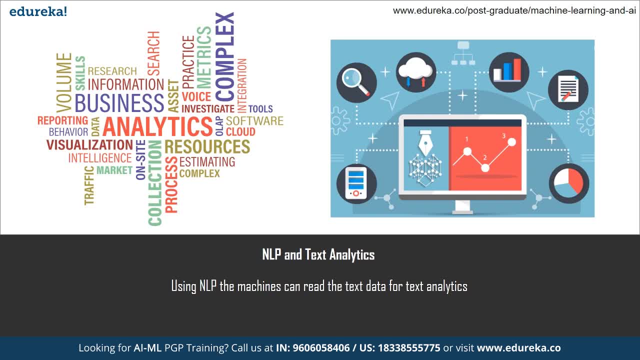 for determining spam in emails as well. guys, and earlier it was quite difficult to build effective applications of NLP and text analytics, But with the evolution of artificial intelligence it has become considerably comfortable and with many open-source applications. One such example is NL TK. 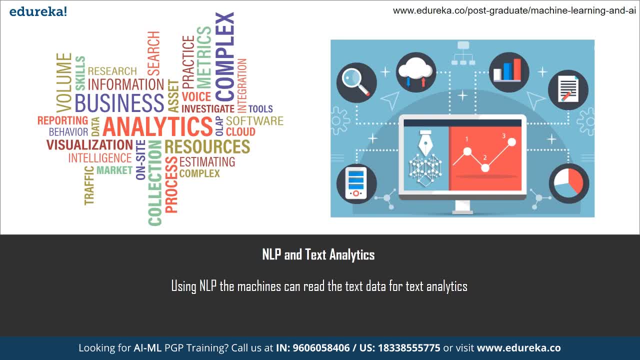 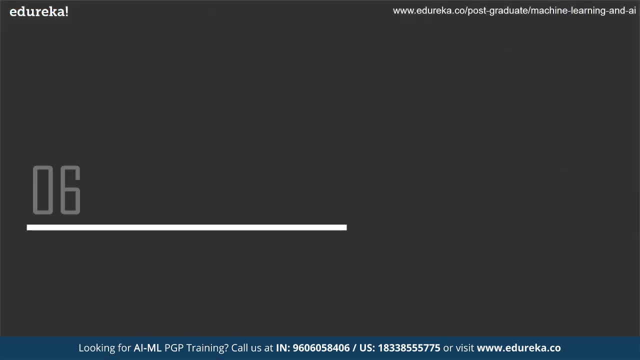 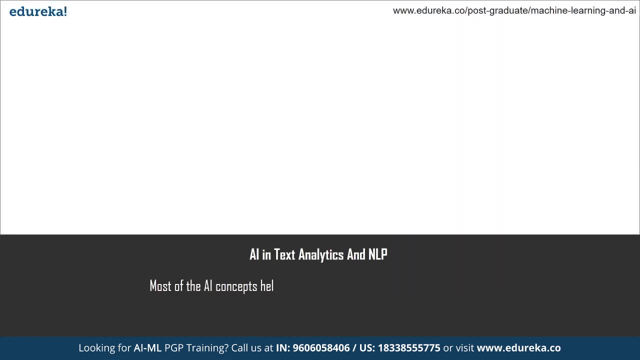 or we also call it as natural language toolkit. And now that we know how NLP and text analytics is connected together, Let us go ahead and take a look at how AI is actually transforming text analytics and NLP AI in text analytics. There are a number of processes. 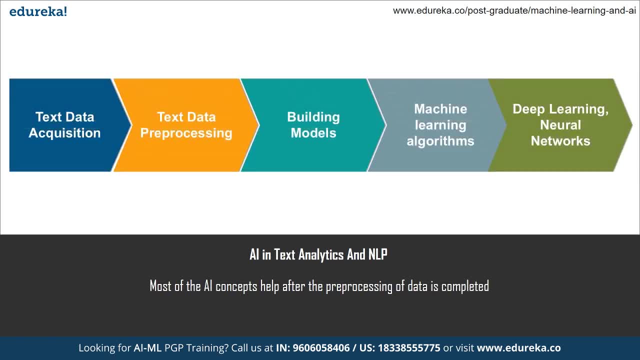 that are required to analyze the text data. all in all, machine learning algorithms are used, in addition to natural language processing, to collect insights for business solutions, such as customer reviews, product improvements, etc. But there are a few steps that are always involved in our text analytics, guys. 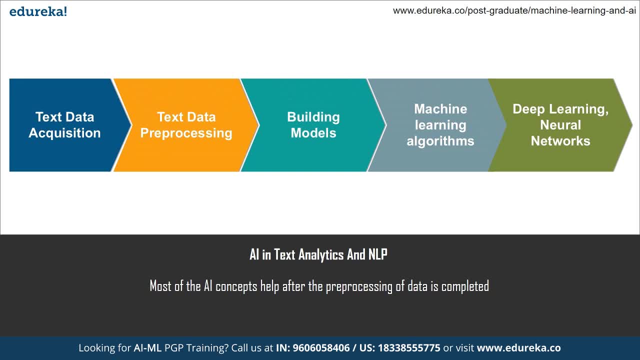 So the first step is data acquisition, or we call it as data collection as well. So text analytics actually begins with collecting the data guys which we want to analyze. So we have to define, you know, select and acquire the raw data, and this can include. 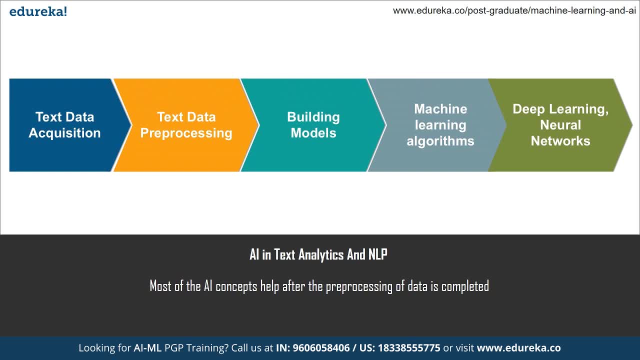 you know, the text documents may have a web pages where we or online reviews or customer reviews and other sources as well. The sources can be anything. first step is to collect the data so that we'll be able to do the next step, which is data preparation guys. 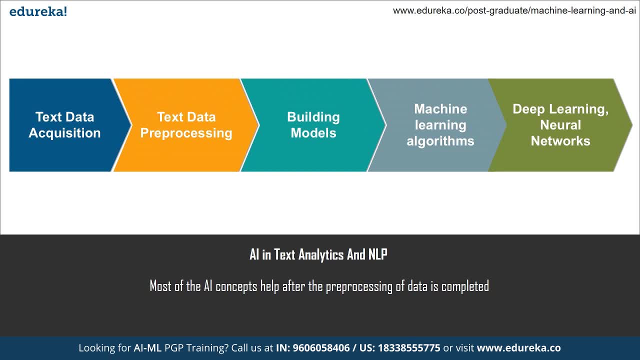 So, once data is acquired or collected, the next step is to prepare the data, for which we have several other steps. So first is text cleaning, guys. This step is actually used to remove any unnecessary or unwanted information, you know, and the text is restructured to ensure that data can be read. 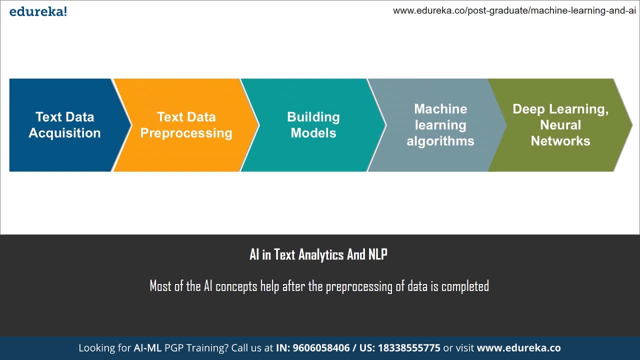 the same way across the whole system to improve the data Integrity, and this is also known as a text normalization. after that, The next step is tokenization, guys, and tokenization actually breaks up a sequence of strings into pieces such as words. There'll be phrases, symbols, other elements and keywords. 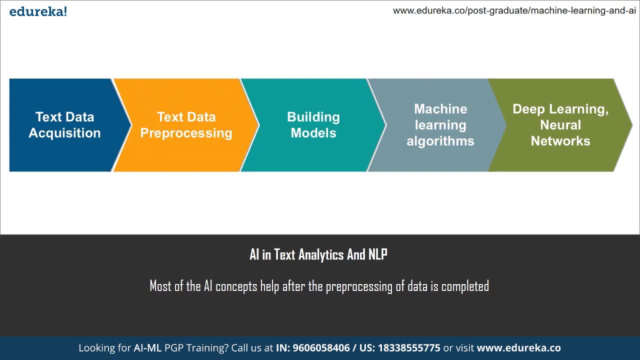 of course, which are called tokens, case, semantically meaning Beautiful pieces such as words, will be used for analysis, and the next step is part of speech tagging, also referred as a POS, which actually assigns a grammatical category to the identified tokens, and the next step is parsing guys. 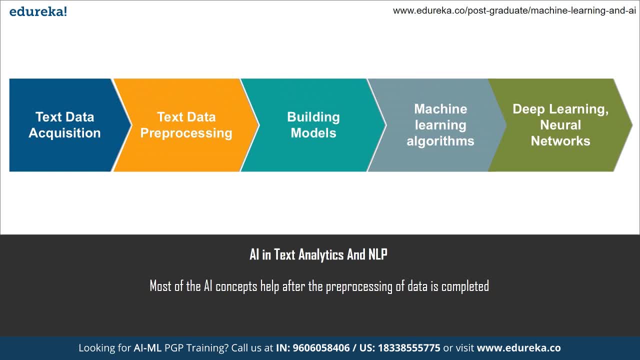 which creates a syntactic structure from the text based on the tokens and POS models. after that comes the third step that we have, guys, which is the text analysis step, guys. So, in text analysis, what we are doing is using the prepared data and we are using the machine learning models that are. 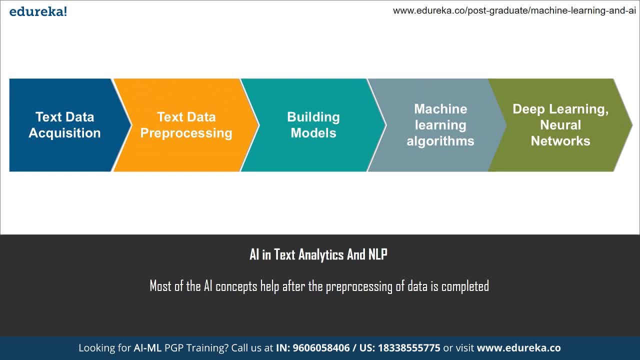 you know, used to analyze the data, and the outcome is typically produced in formats like CSV files, Etc. There can be many ways that data can be analyzed and there are several other approaches as well that we can use, but the main focus here is to use the machine learning algorithms. 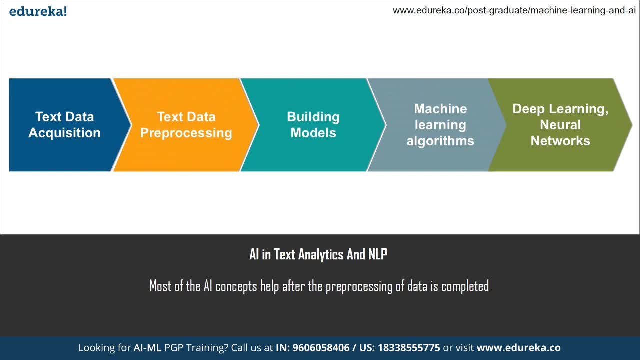 or the machine learning models, in which we use the model to train the data and then after that we test the accuracy and we evaluate the whole stuff and then we are able to get to a point where we have some insights about the data and then we come to the next step. 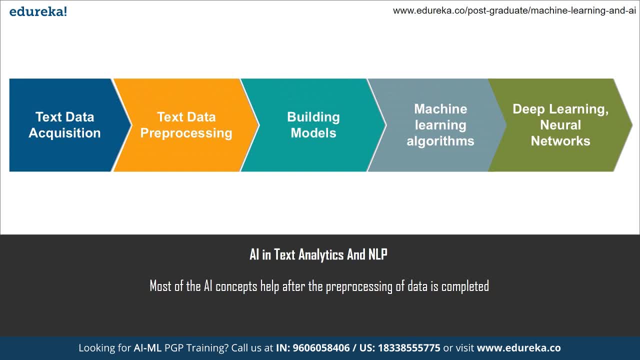 which is data visualization guys. So visualization is the process of transforming analysis into actionable insights. So let's say, after the point of the third step, which is the data analysis, We come to a point where we have several insights, but to put it onto a visualization tool, 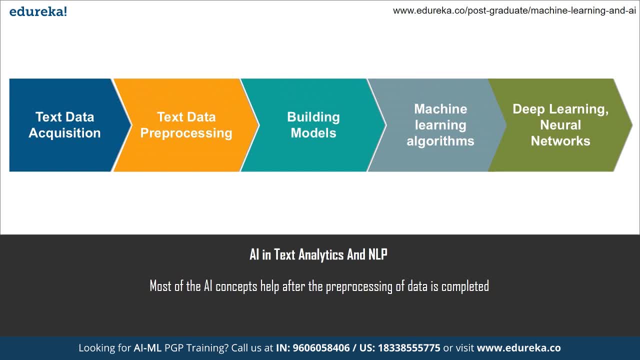 and gather the really important Sites, or actionable insights, that we call them, which are represented in the graphs, the tables, and they're actually. they become easy to understand because when we have a visual representation, it becomes quite easy as- and you'll be able to understand this better in the next session, guys- 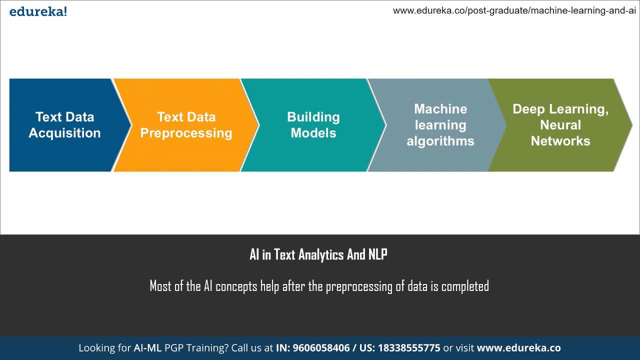 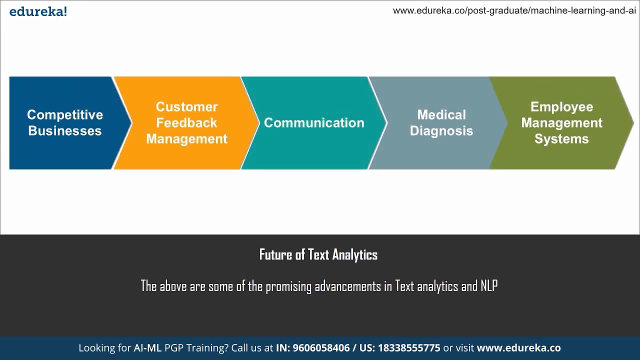 when you're working on the demo with a use case. So we'll move on to the next part here, which is with the evolution of AI in text analytics and natural language processing. the following possibilities has emerged. You can call it as the future of text analytics. 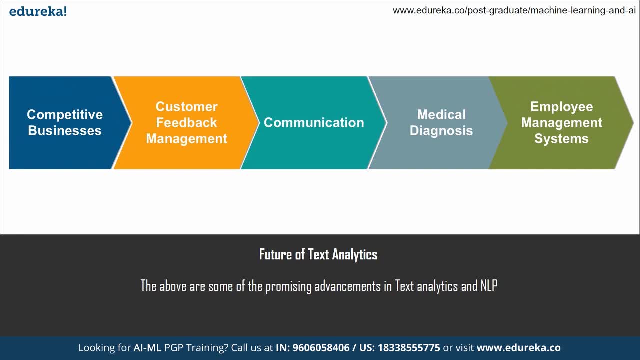 which is actually happening right now also, or in the development process, We'll see a evolution in this as well. So, with the use of neural networks and deep learning algorithms, you know, like neural networks, the convolutional neural networks, the RNN, Etc, or the generative adversarial networks, 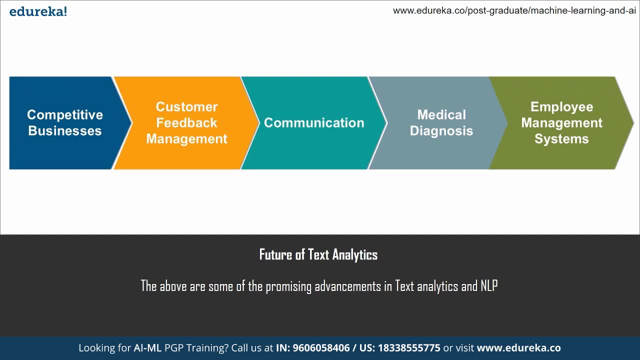 the huge amount of unstructured data can be put to good use into making decision based on analysis. So we'll talk about a few of these future possibilities, guys. So the first one is competitive businesses case. So we'll be seeing a lot of text analytics going. 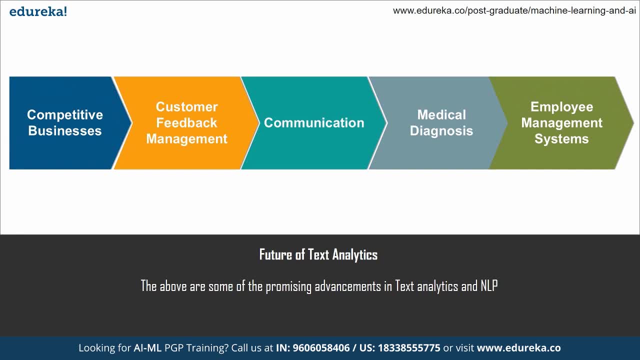 on in the competitive business. Also, you know, we'll be getting a lot of continuous feedback from the customers. like, obviously we are getting a lot of feedback from customers on social media platforms, where they are actually connecting to a lot of people, So there they are actually recognizing the trends. 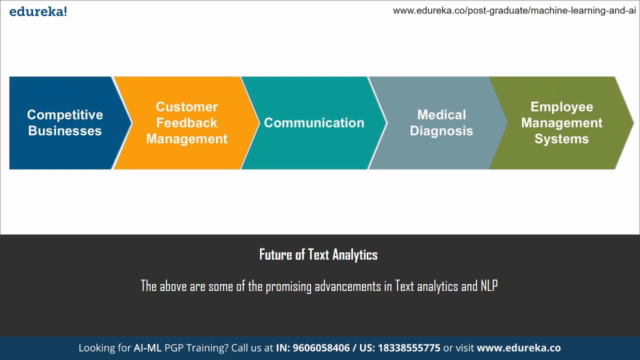 you know what is in the demand and what is not and what is lacking from their end and what are the things that they can do to actually acquire more and more customers. So this is actually creating a lot of demand and supply chain and also creating a lot of competition in the businesses. 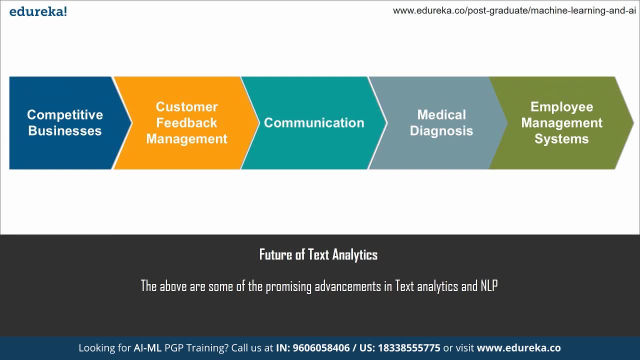 because everybody wants to be on their best foot and they want to produce something that is in the trend that people are actually wanting and through this text- and I'll take- it becomes quite easy for them to understand the insights or the trends as well. Next up is customer feedback management guys. 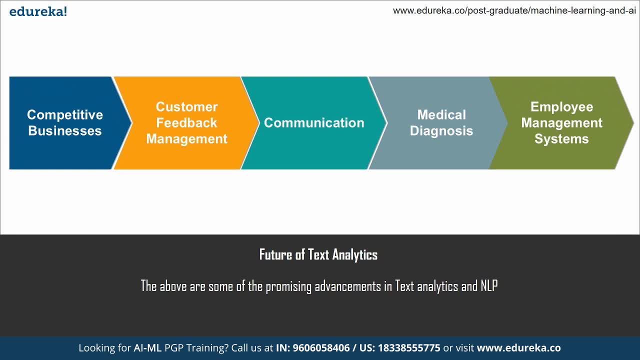 So, as I've told you about this continuous feedback, inside that, there are a lot of things there where businesses are making sure that customers are actually getting what they need, and in inside this customer feedback management, They have the customer service as well. So whenever they- the customer- needs something. 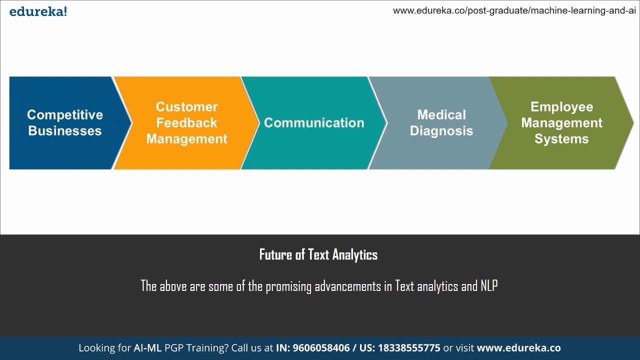 from the business they are able to identify. you know, on a large perspective like this is the main thing that is lacking from our service and we might be able to work on it to actually improve the user engagement or the user experience based on their businesses, Etc. and next up is the communication part. 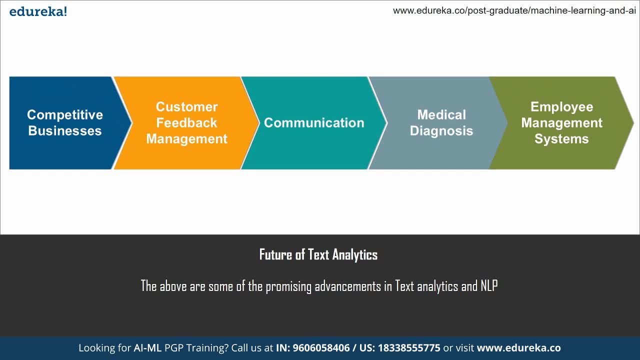 guys in which translation has actually been breaking a lot of linguistic barriers. like earlier, without the text analysis, People might not be able to understand a lot of things that are spoken in different languages, but with the evolution on AI and text analytics it has become quite easy to understand. 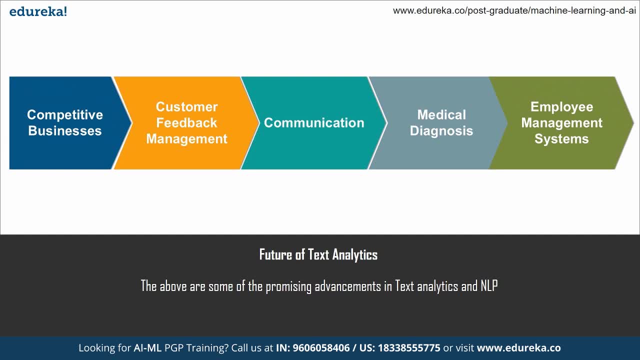 you know, whatever is written in the other text, which is foreign to us, but the machine is able to understand different. It's like you know. it will be able to understand or analyze different languages based on it. It will give us an insight. 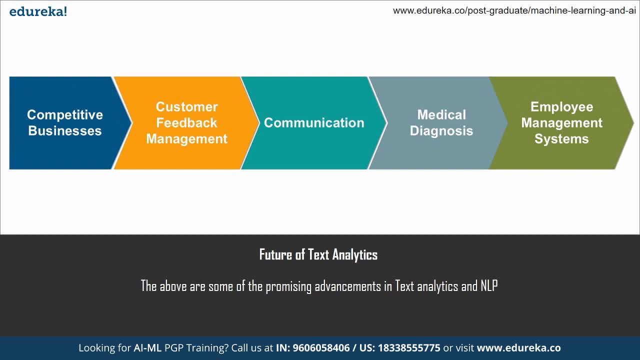 and we'll be able to understand what it means, Whatever text we are getting. one such example is the AI chatbots, So you might be seeing a lot of chatbots. you know where they are able to understand what you're speaking. you know the speech, the transition. they're just able. 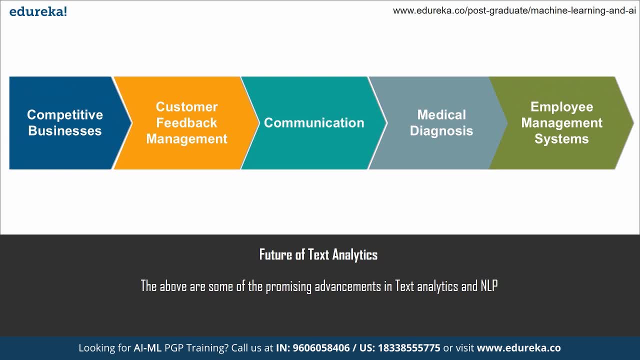 to understand what we're saying and giving you a service. that that is one thing that AI has actually helped in text analytics and a little out of the context. example about this is how an ASL- you know object detection model- where you're trying to put out a hand symbol. 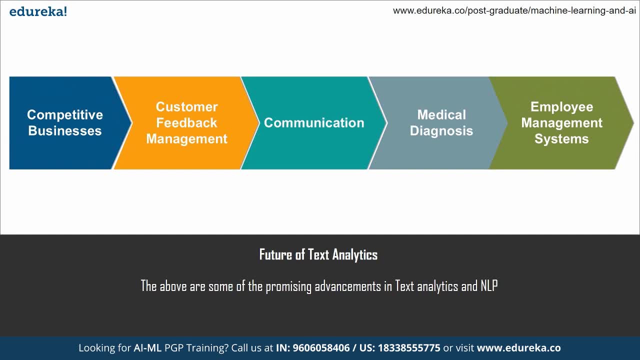 which is American Sign Language, guys. If you don't know about what ASL is, it can play a very good role in communication, guys. We just point to a hand signal inside our camera and it's able to convert it into- you know, speech, guys, or maybe a text where you'll be able. 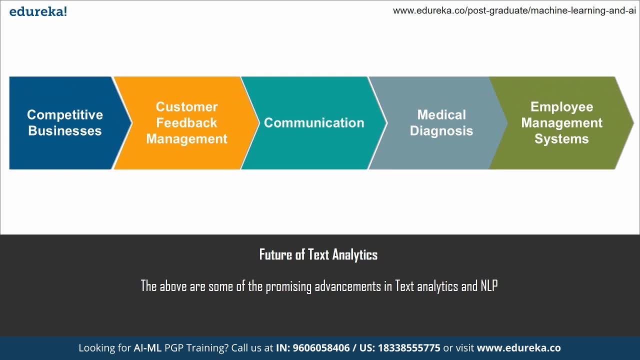 to understand what the other guy is trying to say, because most people does not understand the sign languages. This is a little out of context, but I'm trying to tell you how AI is reshaped, Shaping the communication, and in which we have the natural language processing as well. 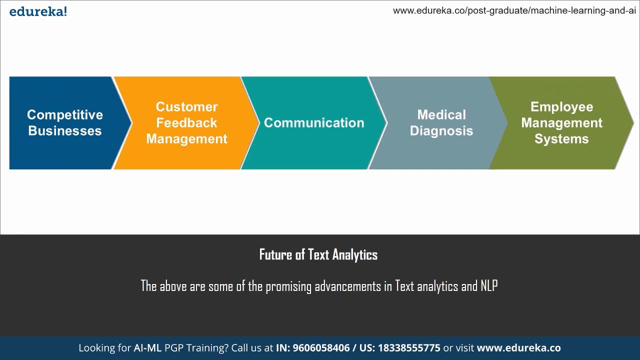 and recognizing the patterns of distress as well. I mean, if you take a look at several posts a person is making throughout the year, I mean, let's say, if a person is tweeting for every day for the whole year, if we look at the pattern, recognize 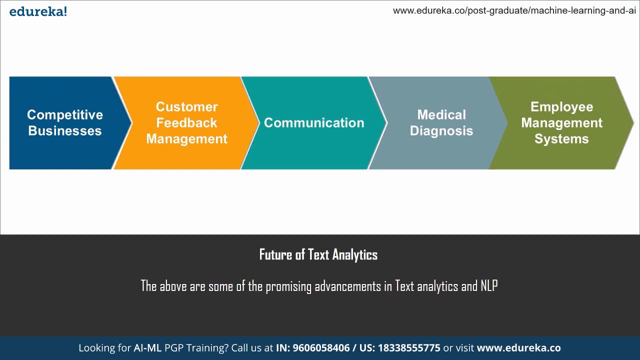 how a person is trying to think, what kind of forces in making, recognize the sentiment and trying to get the insight. So there might be a few possibilities that we are able to understand the psyche of the person, How he's trying to understand the stuff or what he's going through. 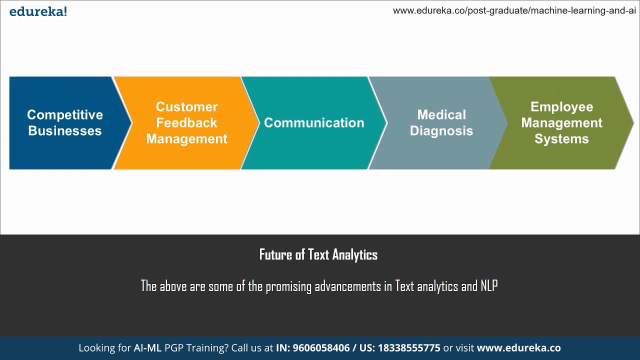 and what is trying to convey with the post that he's making, and by studying the past communication data. of course- and there's just an example, guys, We are going to need a lot more data than that, But this is just in a possibility that I'm talking about. 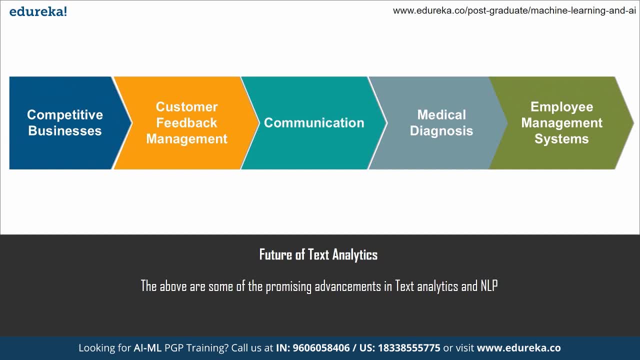 and then there is medical diagnosis. Of course, guys, if you have a lot of previous data or the text data we are able to analyze, it will be able to understand the diagnosis, guys, because most of the cases that we have in a medical Profession, they have similar patterns, guys. 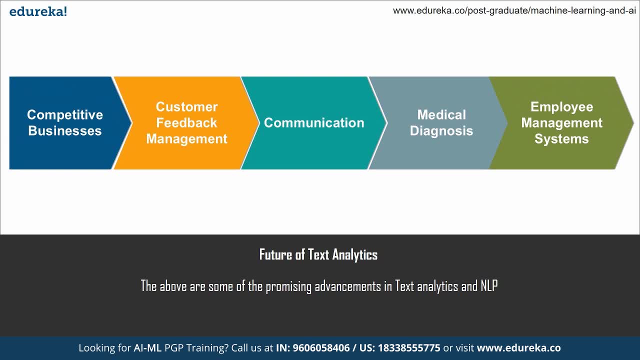 in which kind of difficulties that they are facing in life or the disease that they have. the symptoms might be quite same and they might need the same kind of medicine. Sometimes, of course, it has to be gone through a doctor first of all, but medical diagnosis is actually benefiting. 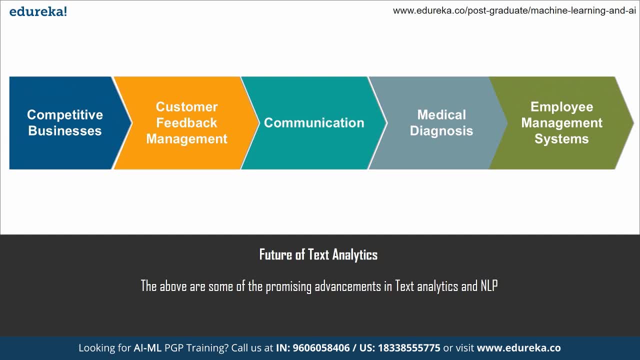 from text analytics because they are trying to make it as a thing, guys like, if a person is talking to a doctor on phone and using the speech to text module in AI, they are able to get everything on text. So by the time you're done talking to the doctor.